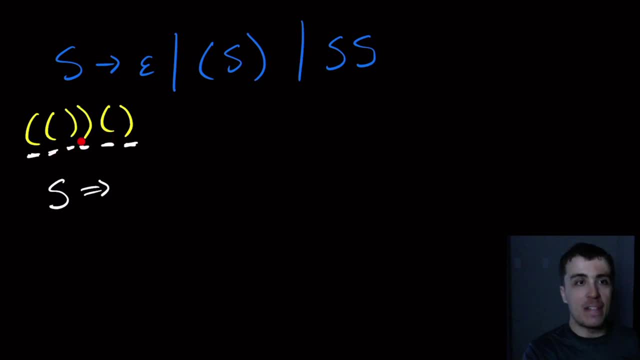 So I can apply that right parenthesis over here. but the stuff in the middle is not balanced on its own, So I need to apply the SS rule right here. So then this, the left S, is going to generate this left half of the string, And then this S is going to generate this right half. It's not necessarily the half, it's the second part, because these variables are independent of each other. They don't have to generate exactly the same length of string or the same string at all. 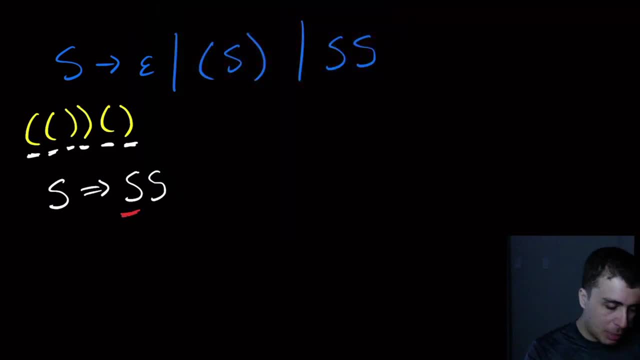 So let's work with the left S then. So I have the left S and I want it to generate the left half of the string, the left part of it. So the only reasonable thing that we can do, because we have this nesting of lefts and rights here, I should apply this rule twice, Because if I apply this one then I don't have that structure over here. This is the only reasonable one I can do, So let's apply that one. So we have left S, right S. 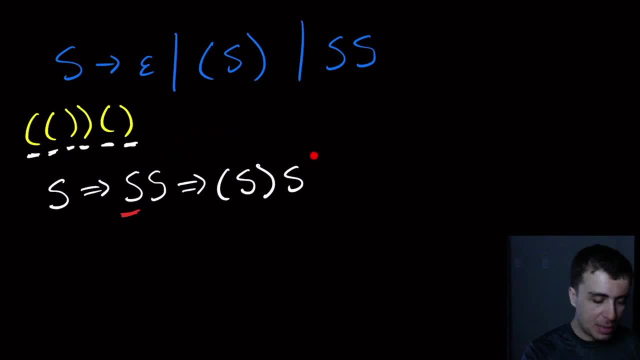 So this second S is the same as that one, But this one is just applying the rule on that S. So, effectively, effectively, that S got killed off And we got it here. So then now I'm going to apply the same rule again to the left S here, So that S is going to go away And what we're going to have is left, left S, right, right S, And then now, since we have the two, 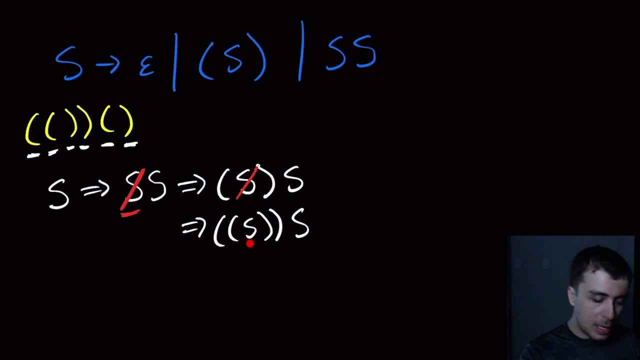 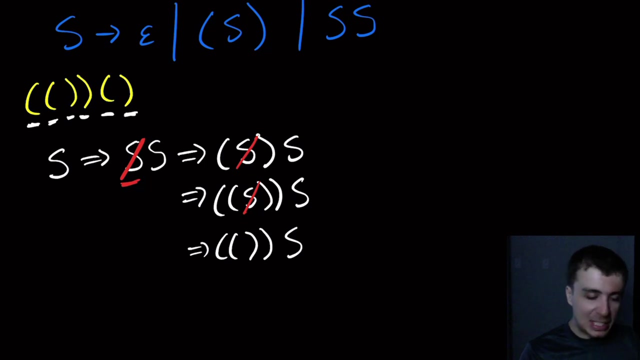 nested parentheses or set of parentheses here. I want this S to go away because there's nothing in the inside here. So I'm going to apply: S goes to empty, which is one of those rules, So that S is going to get killed off, And then I'm going to get left, left, right, right S, And then it's pretty obvious what the only variable S is going to do at this point. So we're going to kill that guy off And then now we're going to 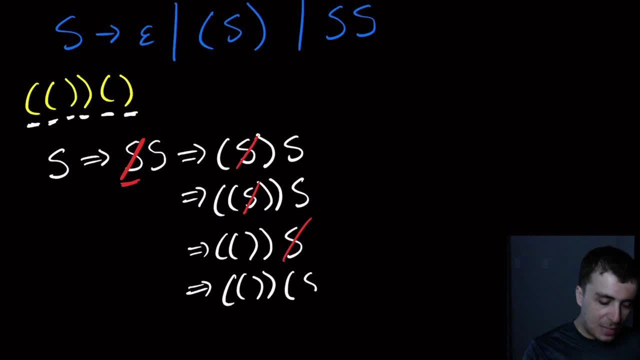 apply left, left, right, right, left, S, right, And then one more rule application where we get rid of that S, And then we're going to have that S go to empty, because that's one of the rules. So we're going to have exactly what we would expect here, which is pretty cool. So it's. you can kind of see what's happening, right? You can see, okay, we're replacing that thing with stuff, And then we replace that variable with stuff. replace that variable with stuff. 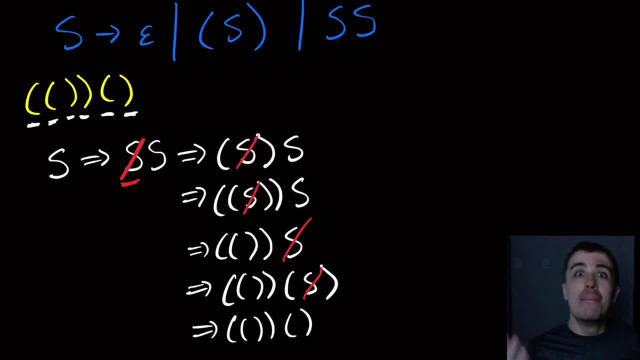 variable with stuff, replace it with stuff, replace it with stuff. but it's not really a visual thing and you can, because i arranged it this way. it's kind of visual but it's not really like a picture where you can actually see what's going on. so the way that a parse tree works is that what we do is? 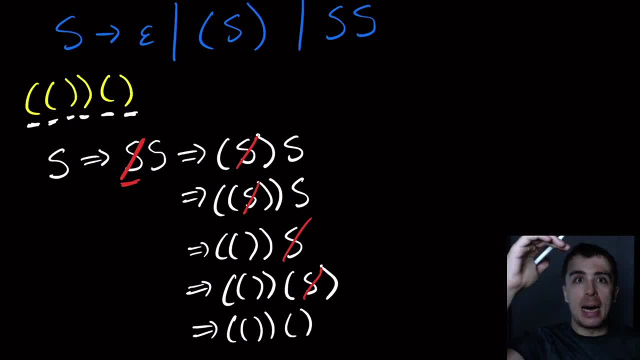 we start with the start variable at the top and we apply a rule, like we did here, and those things that are, as the result of the variable, being replaced with stuff, appear as children underneath. so what do i mean by that? what i mean is: so this s right here. that's going to be the top of the tree. 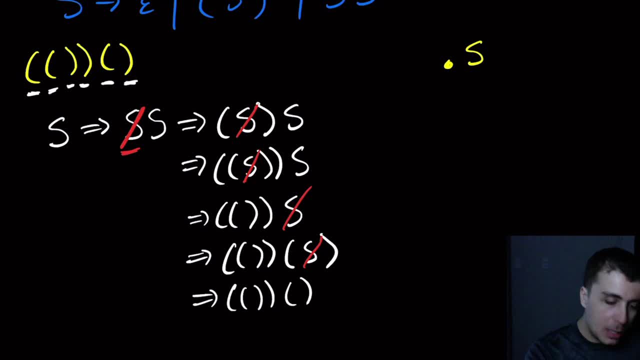 so let's, let's make that the s up here. i don't know why computer scientists want to have trees that grow down. you know they're not going to grow down. you know they're not going to grow down. you know they're not going to grow down. you know they're not up, but anyway, that's the way that. 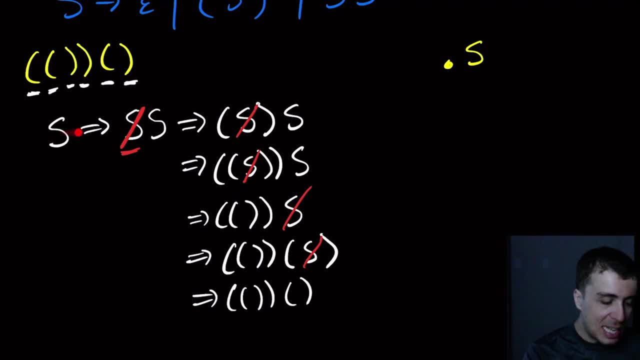 this works. so here we replace this s with two s's, so the children underneath this are going to be the result of what the rule application was, which is replacing that s with two things which are s's in this case. so the children underneath here are going to be one s and then the other s and the. 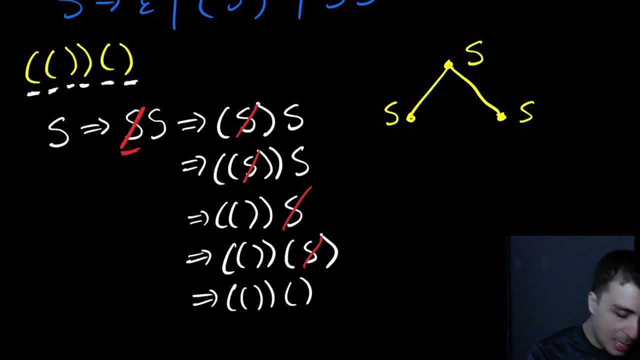 second is: this is going to be one s and leave twice, two putsch. okay, so we need a two letter to a DAY line. so here's that question. that question, is, is wrong. this is from the article about the s and the smoke tree. read it left to right. of course you can define it as reading right to left, but this is just the convention. so this s is going to be the one that we replaced on the left. so the화�ibly. we read that left signs up on white and the s will always be the right sign on these parts. 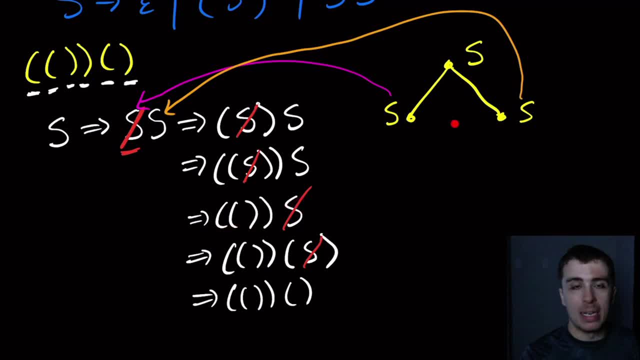 left, right here, which makes the, the double nested one here, and then s on the right side here, is gonna make the two little parentheses on the end. so what we do is this s right here, the one that's being pointed to in pink was replaced with left s and then right, so then those are gonna appear as children underneath. 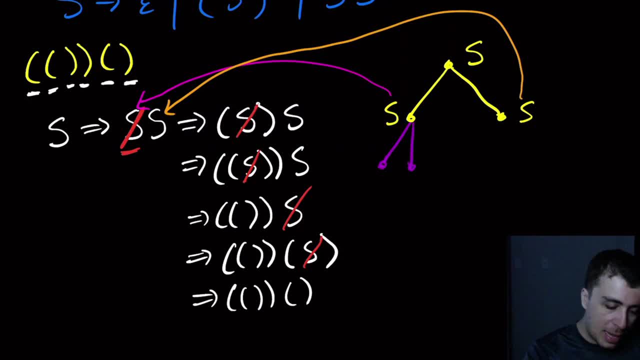 that s. so this is gonna have three things under it, because we had the left parenthesis, which is a terminal s, which is a variable, but a variables can appear as nodes in this tree, and then we have the right here, so then we have. so the way I'm gonna notate, this is left and then s I'm gonna try to fit in there and 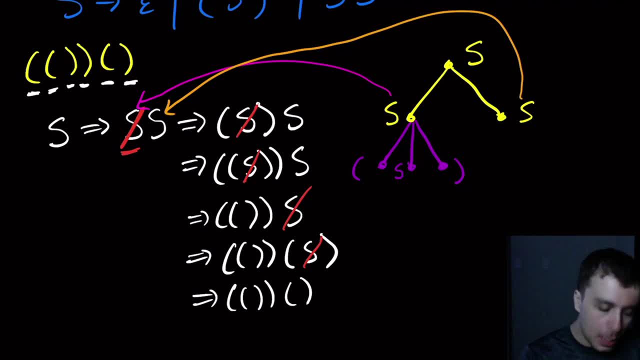 then right parenthesis. so here the nodes right here that correspond to the left and the right parenthesis. because they are terminals, they're not gonna have any children under them, because it's a context-free grammar. we can only replace a single variable with stuff. we can't replace a terminal or anything else with with stuff. so but this s. 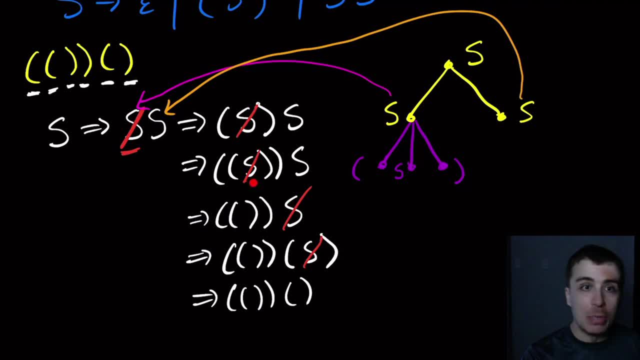 because we had, we replaced it with stuff that's going to, namely this one right here. in fact, I'm gonna draw a line, so this s right here is gonna be that s right there, because the pink one was right here, and then the one that appears underneath is the one that appears. 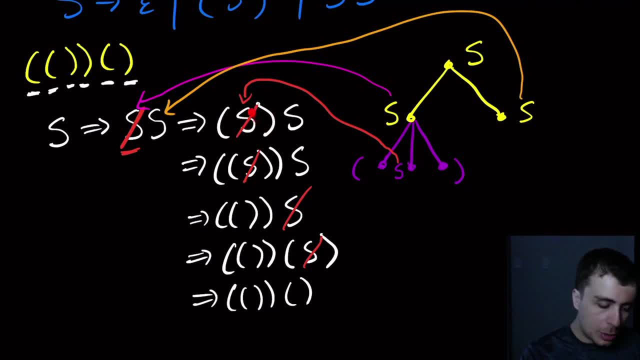 immediately the rule application afterward. so then that that s is right there. well, we replace that s with left s and then right. so then I'm going to have left s and then right. so then what we can see is that this s that we just made is that s right there. 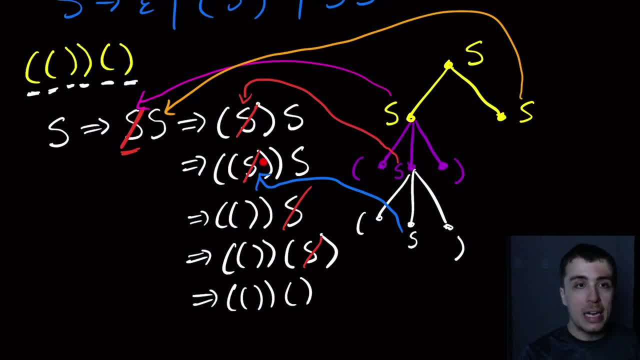 and we notice that in this rule, right here, we replaced s with empty right, because that's one of the rules that we applied. so then, the children, the child underneath this one, you may think: well, it was replaced with nothing. so what do you do here? what we do is we actually put the empty string as a, as a node in. 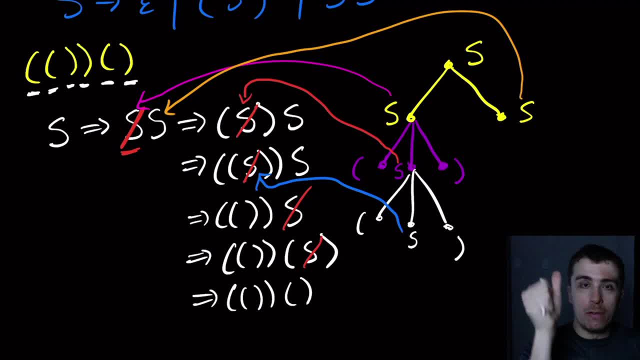 this tree. so the things that can be nodes in this tree are variables, which are clearly here terminals or the empty string, and and those are the only things that can appear as nodes. so the node under here is going to be the empty string, and that's to symbolize the fact that we 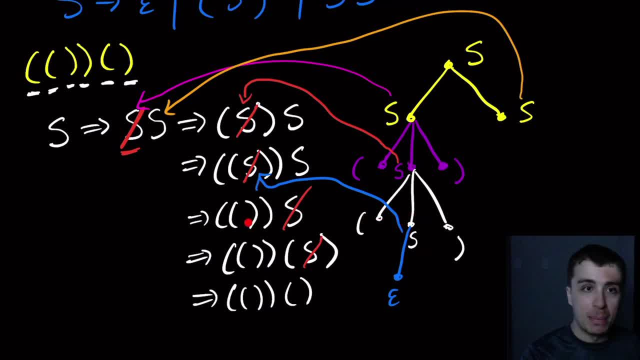 replace this particular s with empty. so then, over here, what are we gonna do? well, this s, which is this orange one being pointed to, is the same one right here is the same one here. now, here we replace this s with left s, and then right, and 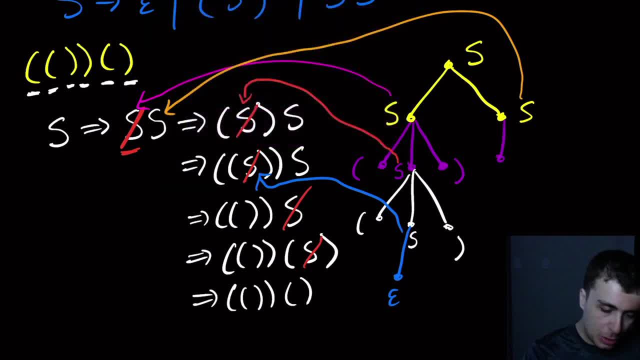 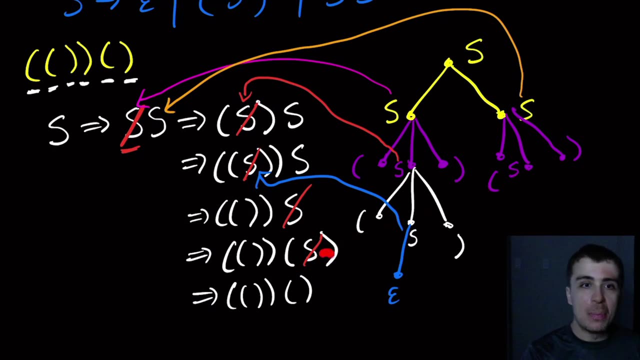 so let's go ahead and make that substitution, so we have left, and then s. maybe i should move that s over so i have some room and then right, okay, so then this s right. here is the one inside the parentheses, right before the very end: right here and right here we were. we applied s goes to empty. 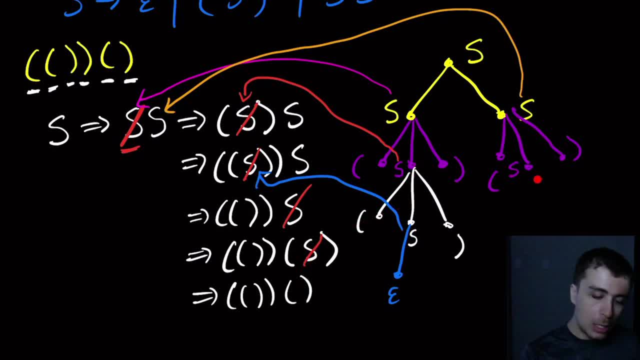 because there's nothing inside the parentheses anymore, so the child underneath here is going to be just the empty string. okay, and so this is now a parse tree for this derivation right here. so remember it's a derivation if we start with the, the start variable, and end with a string only. 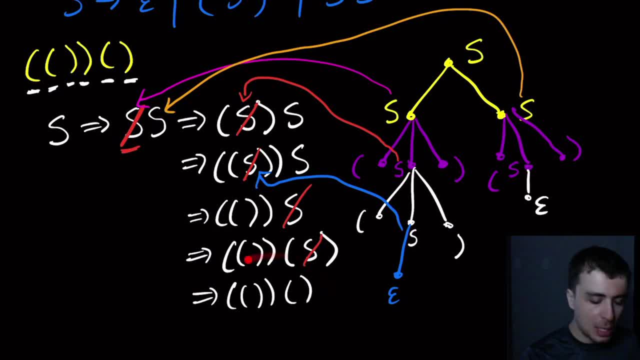 composed of terminals or the empty string. i guess which is what we get here? well, do we actually read this parse tree? well, what we do is we read the nodes left to right. uh, read the leaves from left to right. so if we read the leaves left to right, well, the the leftmost leaf in this 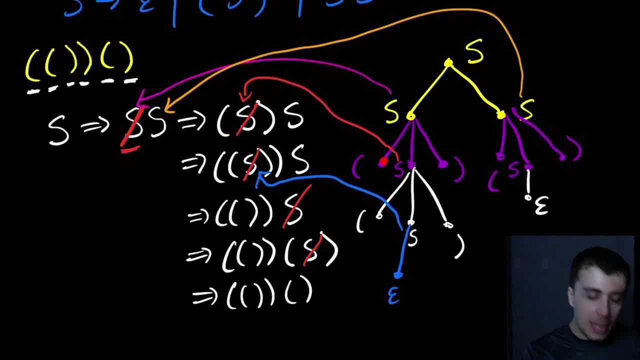 thing is that node right there. and then what is the next leftmost node? which is this one? and then, uh, this one right here is the next leftmost one, leftmost one, next leftmost one. and then we come over here, here and then here, so effectively we're just reading the leaves from left to right and 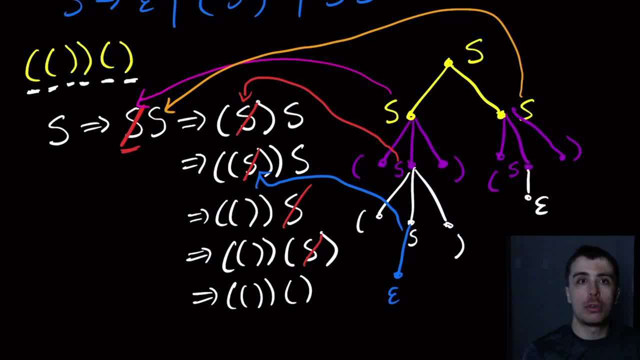 then now we can reconstruct the original string using this particular representation. it's a different representation for context-free grammars in their derivations, so you can deal with grammars in this way and it's it's more formal. i agree. i see the value in having a derivation because it's 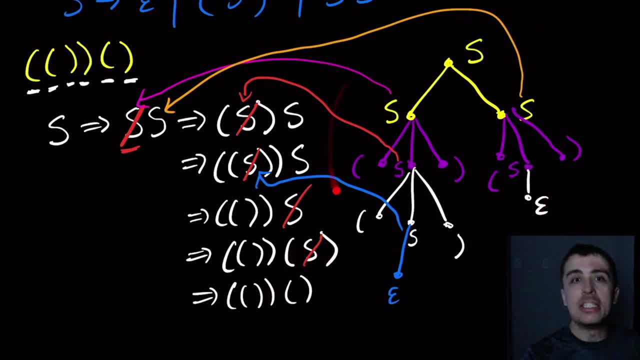 incomplete. it's not completely formal. however, it's a lot easier to think about what's happening right here, so we can actually see the derivation happen just by going from the top and working your way down, because the things that appear underneath a node are the result of applying a rule to that. 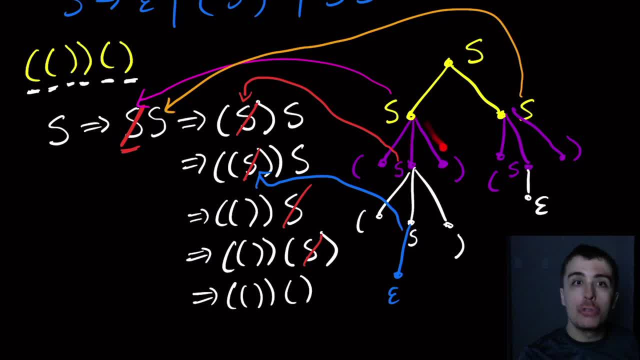 particular node, and we know that if a node has children underneath it, it must be a variable, because it's a context-free grammar. you can only replace a variable with stuff. you can't replace anything else with stuff, and so that is what a parse tree is: it's a visual representation. 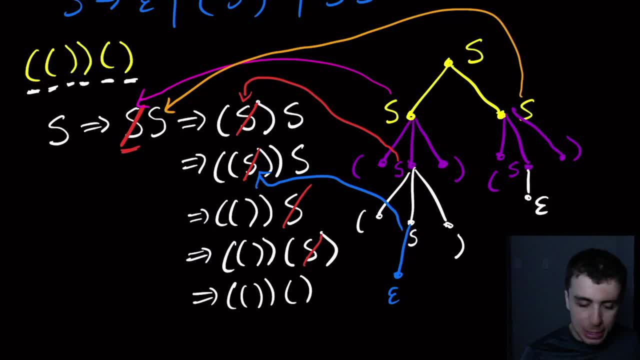 of what a context-free grammar is doing. what is the use of this? well, you can prove certain things about what a grammar actually does. so what you can prove is that, since this just as an example- so look at this node right here, so there's an s obviously right here and there's an. 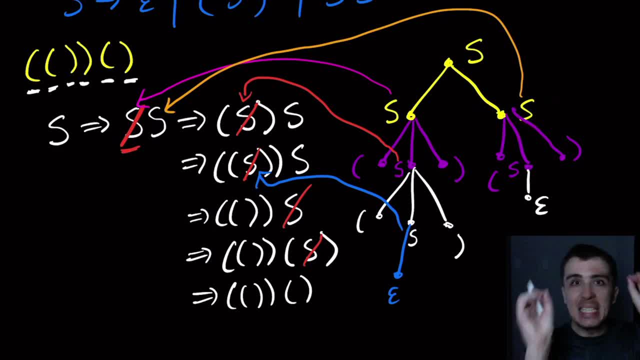 s right here. so what we can notice is that it's the same variable in both places. so because it's the same variable, i can copy and paste this sub parse tree over to here i can. i can copy and paste this sub parse tree to anywhere where there's an s, because it doesn't matter what's around. 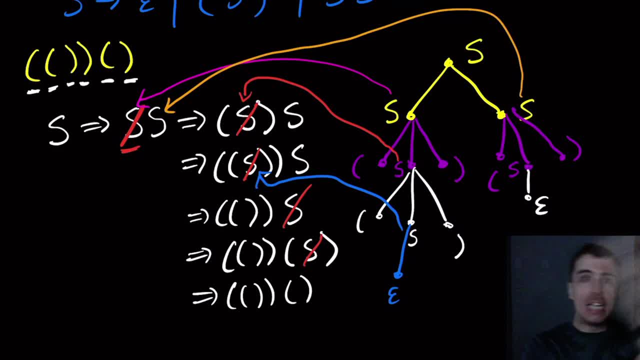 the s in the derivation. i can just copy and paste the parse trees around, where it's a lot harder to see that over here, because you have to kind of know: okay, i'm right here and i have a bunch of s's in my derivation, where do i actually copy and paste and what do i copy and paste, whereas here: 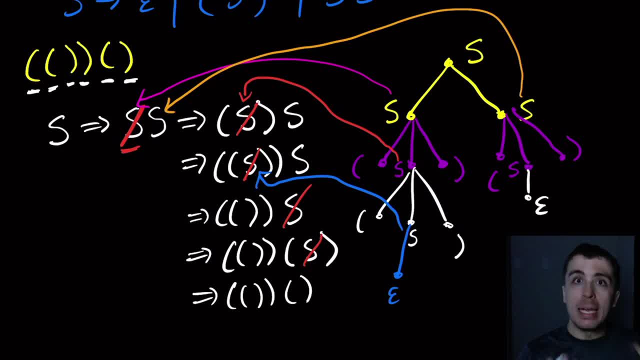 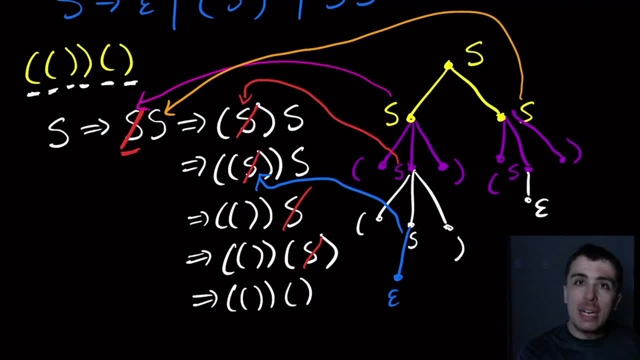 it's a lot easier to see what's going on. so here we can actually figure out from some parse tree what other strings can also be made. and another amazing fact is, if you have a parse tree force string, when you read it left to right, that string must be able to be generated by the context-free. 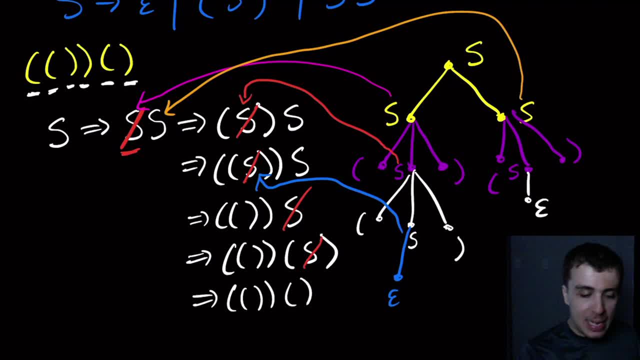 grammar. so, and the reason for that is, you can verify whether it is it. let's just say that we don't know whether this string is generated by the grammar. well, we can see it just by going from the top down, whether or not each of the rules was correctly applied and if there wasn't. 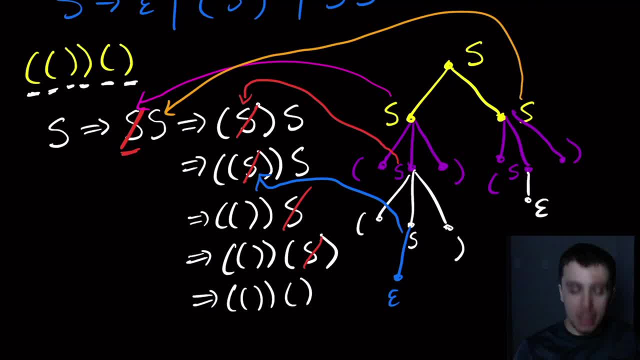 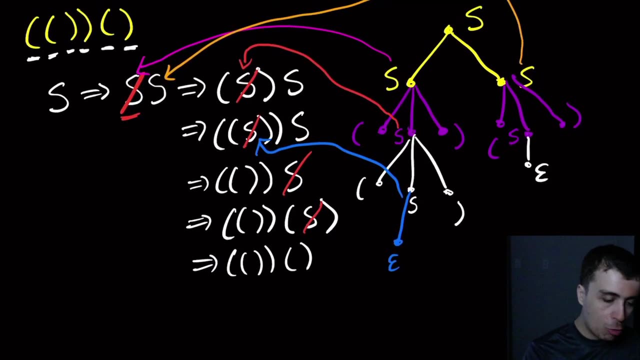 one correctly applied, then we know that it couldn't have been a valid derivation and that, and if you have a string that um is not in the language of the grammar, it can't be made by this parse tree. so therefore, that actually tells us something really, really important. 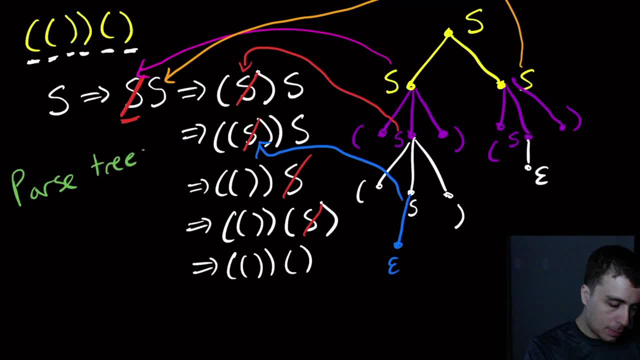 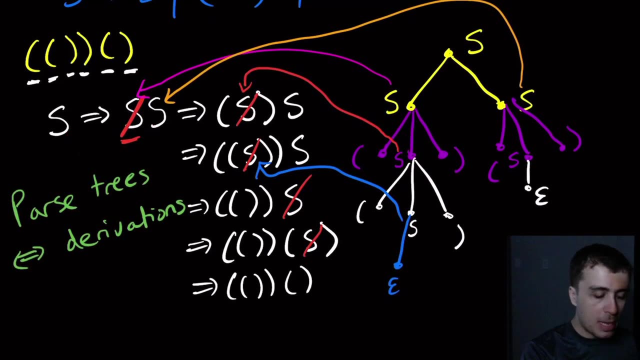 which is that parse trees are in some sense equivalent to derivations. so if you have a derivation for some string, you can convert it into a parse tree, because you can just do the same procedure that we did here. whenever you apply a rule, you put children underneath the variable that you replace stuff with, with the 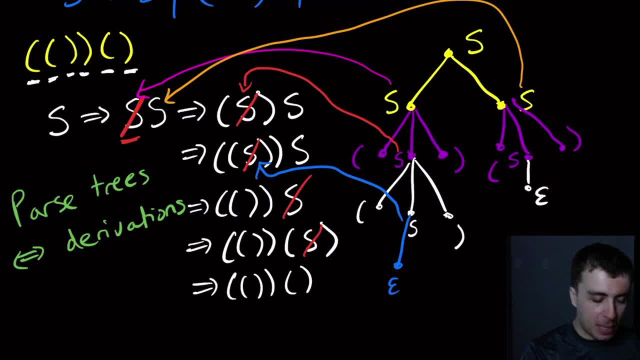 stuff that you replace with. if you have a parse tree for something, then it turns out that you can actually have multiple different derivations, because here there's no um, because it's context free, uh free. here we could have worked with this s first instead of this one, because